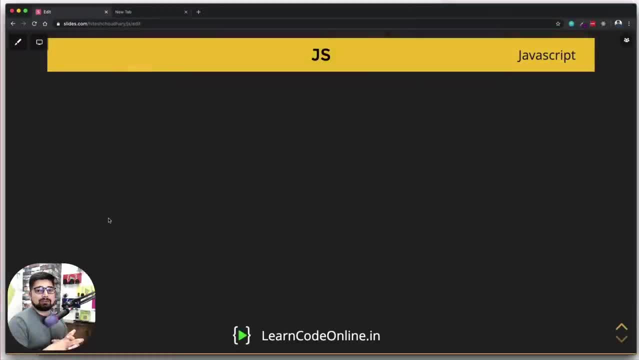 scene so that you can relate things with the real world implementation of the stuff. This is going to help you a lot in understanding the things. Also, I will be calling up LearnCodeOnline as an app- and it's not just about mobile application, Anything that's in the computer. 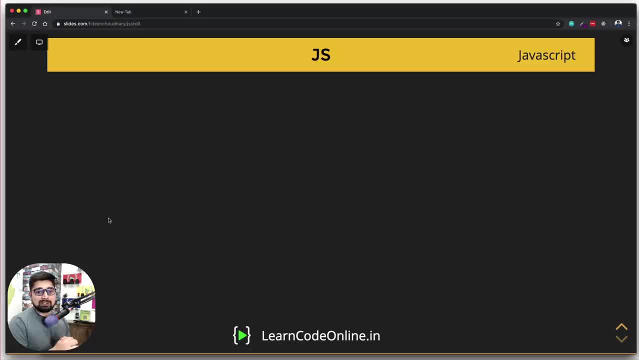 and that runs and do something is known as app or application, and application doesn't always need to be in mobile. Anything that runs on the web as well, or browser, it's also an application running in the browser. It can be running up inside the console as well. 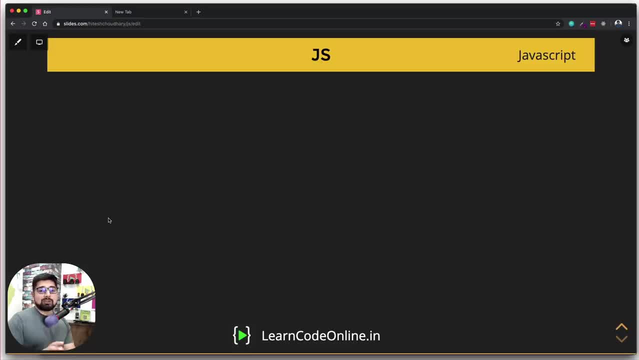 Simply a command line, app or application. So, in general, for the new people who are just trying to learn programming for the first time: yes, I will scatter this word all around the places calling everything as app or application, So please keep that in mind. Ok, So let's just say you want to. 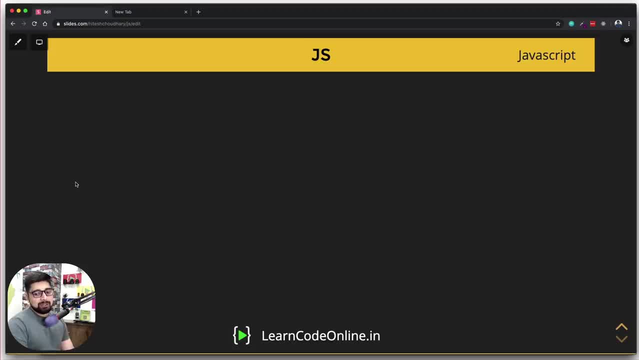 build an application which is almost similar to LearnCodeOnline. So what's going to be your first thing? First thing is: I want to reserve some space in the memory, And by that means let's go ahead. memory in the reserve, some space in the memory, also known as declaring your variables. now we 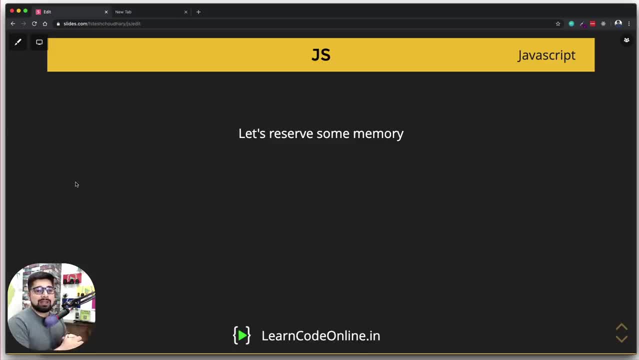 have a whole lot of varieties that how these variables can be stored- some permanently, some not so permanently- and whole bunch of other things goes on around. but right now let's just focus on these three keywords and eventually we're going to talk more about this as we move further. the 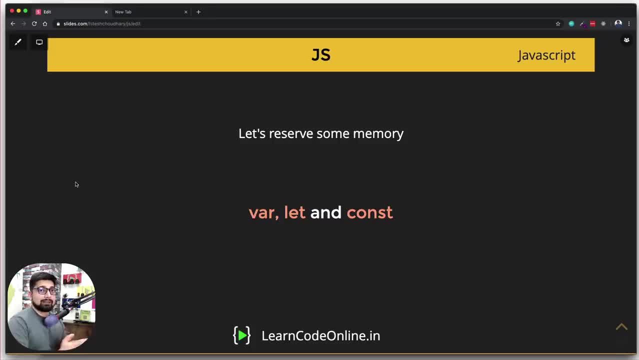 three keywords you're going to see is war, let and const. again, they are very different and their working flow is very different. the most common that you're going to see all around is this: war keyword. war simply means I want to declare a variable and this is going to store some of the 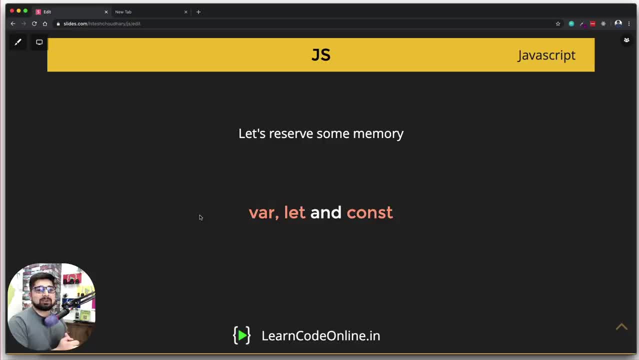 keywords there, for example in the learn code online. I want to use that. what is your name or what is your email, what is your password? these things need to be stored somewhere and for that, in general, we're going to use war. another keyword is there for similar purpose, which is: let and we. 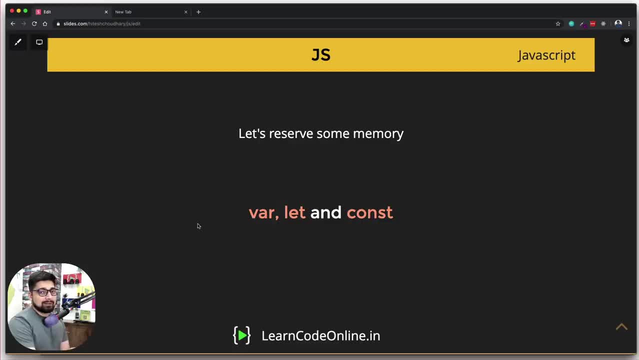 cannot understand the difference between war and let just right here, because a lot needs to be understand for that. so let's go ahead and see that, how the this war can be used. now let me open up my vs code and we're going to discuss that there. so this is. 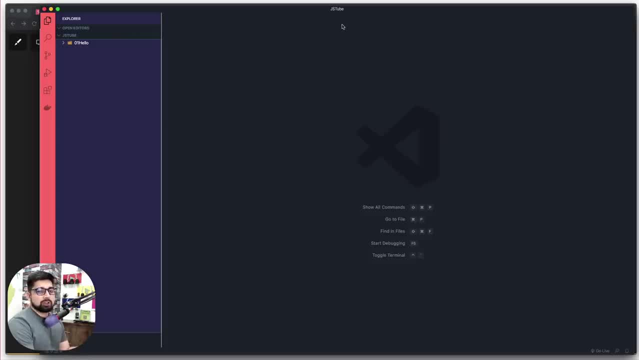 my vs code. i have opened up my entire folder here, which is js tube, and i'll keep that as an attachment so that you can check it on my website as well. all the files will be available there, and i'm going to create a new folder here and i'm going to call this one as zero. two basics we will. 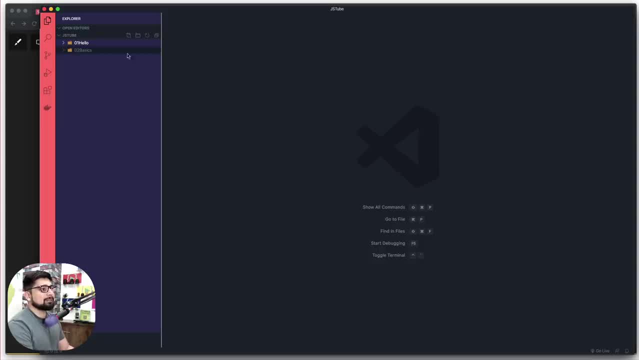 be creating a bunch of files in this, so it's good way that we keep all of them in the separate. i'm going to open this up and i'm going to call this one zero one, and i'm going to call this as variables, and, of course, don't forget the extension, which is dot js for javascript, and we will be. 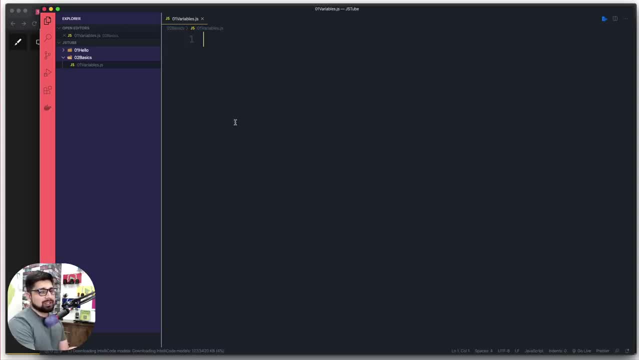 running from now onwards the application using node, because it's much more easier. i don't have to attach it on an html, i can just directly discuss whatever i want to discuss. so the simplest way of declaring the variable. there is no such thing as in case you are coming up from c or c plus plus. 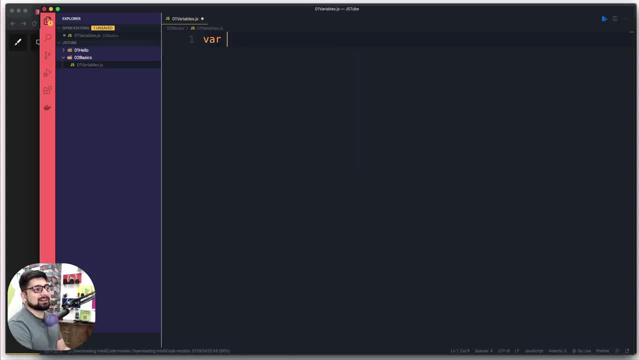 there is no hash include or something like that. there is nothing. you just directly start writing your code in javascript. for example, if i just say that i use your full name or i want to store the user's full name, i'm going to go ahead, use the name full name and then come up simply with the double quotes i want to. 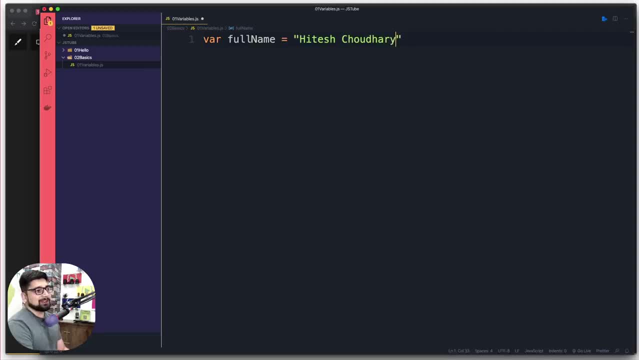 store this one, so i'm going to write my name here- you should be writing your name by now- and followed by it, you can place a semicolon here. now, javascript is very forgiving about these semicolons, but for good practices, we're going to keep this. now, this bring the the simple conversation about how to. 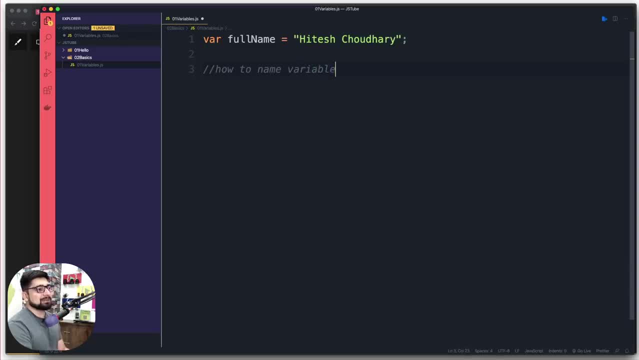 name variables. this is a big subject and people like to discuss a lot. the way how you can define the full name can be a couple of ways. you can simply say like this: what i said full name. or you could have said something like this: you could have said full dash name. or you could have said something like full underscore. 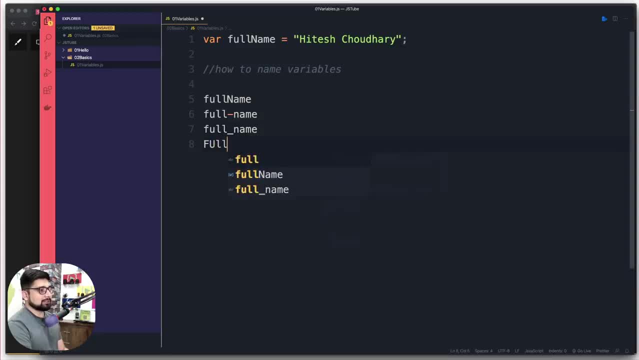 name and probably you can say something like this: full, full name. so which one is the correct and which one is the best practice that you should go now? first and foremost, i would like to discard this last one here again, due to good practices. there is nothing to do is. this is not going to give us any error. first and foremost, whenever you name: 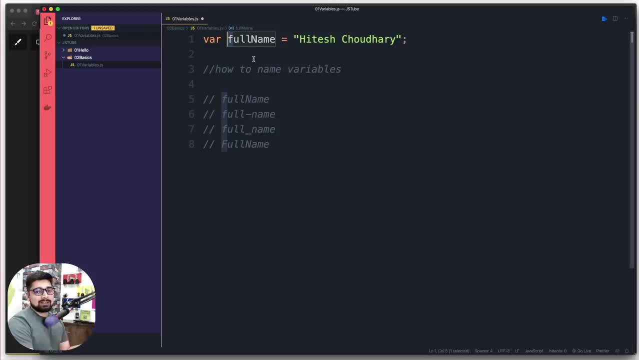 anything. you should not start a variable with the uppercase letter. it's generally not a good thing. it's not going to give you any error while defining some classes and all other great things. we just use this uppercase letter, so there's a specific place where we use it. apart from this, for these. 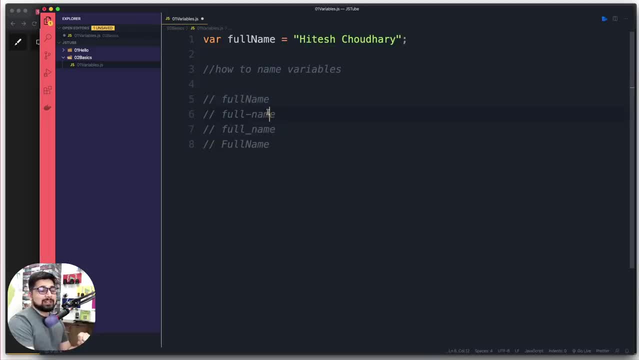 three things. i have no problem at all and i have a good reason to use this uppercase letter, because you're going to see that people say that this is what you should use, but people also will come and say that you know what you should use: dashes to separate your and make your variable more readable. 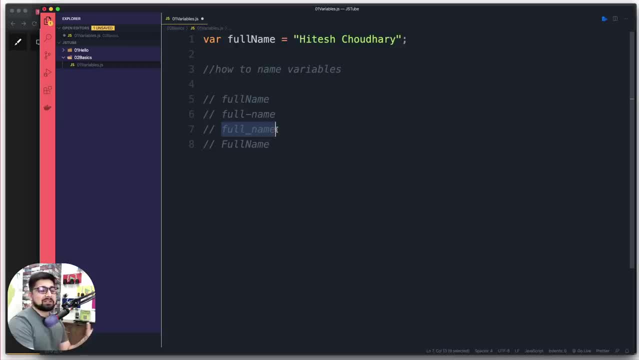 as the name. some people will say: use snake case. yeah, these ones are known as with a snake case. this one is also known as camel case, so which one i recommend? i would say there is no recommendation here. just make sure whatever you're using, stay consistent. don't just use snake case some places. 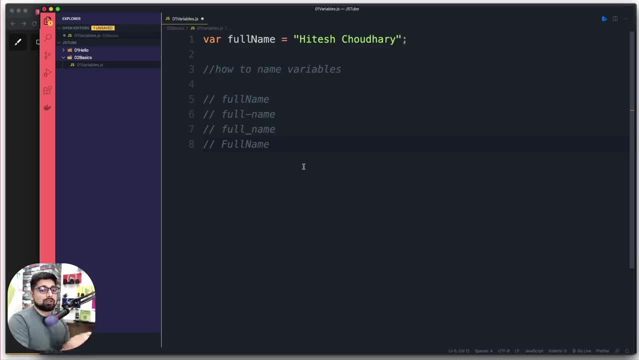 some places camel case. that's a bad thing to do. just make sure you pick up a style and stay consistent with it, and that's it. that's all about it. i usually prefer to use these camel cases because i think they are much more readable, so that's what i prefer. but in case you are a big fan of using snake cases, like you, with the underscore. 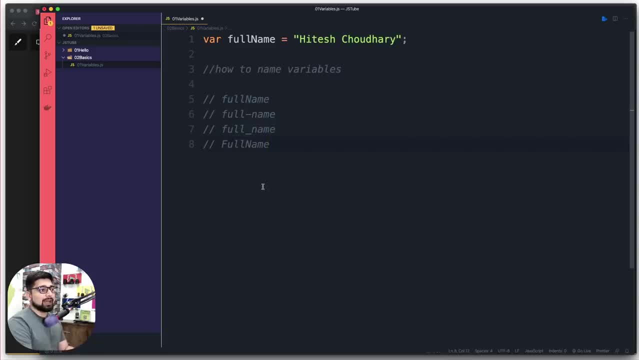 you can stay with that. no problem in that. surely you're going to have to argue with some kids. that says no, this is for javascript, and in c++ we use underscore. there's a lot of kids around here, so don't worry too much about them. as long as you are consistent, that's all that matter. okay, now you. 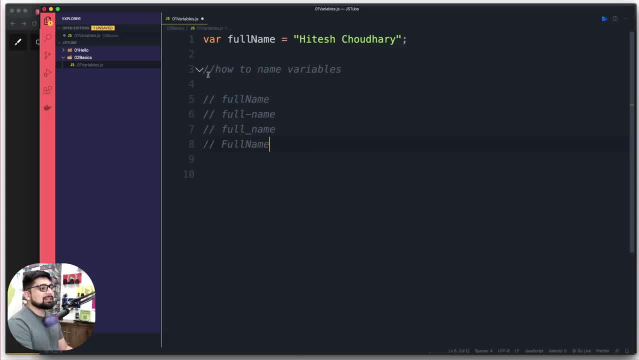 might have noticed that i have a lot of kids that are using snake cases and i have a lot of kids that are using snake cases, and i have a lot of kids that are using snake cases and i have a lot of kids. that is that i'm putting up. is these double slashes here? these double slashes are simply means that 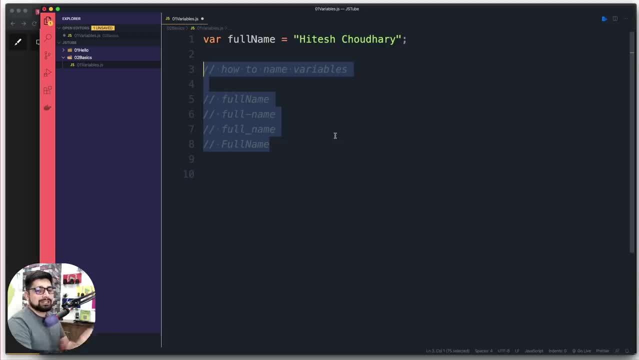 i want to comment out this code. this code will never be compiled or turned into the machine code. this is just for my own reference and there is a quick shortcut for that. you can select a number of lines and use control slash if you are on a pc. if you are on a mac, command slash, so it just 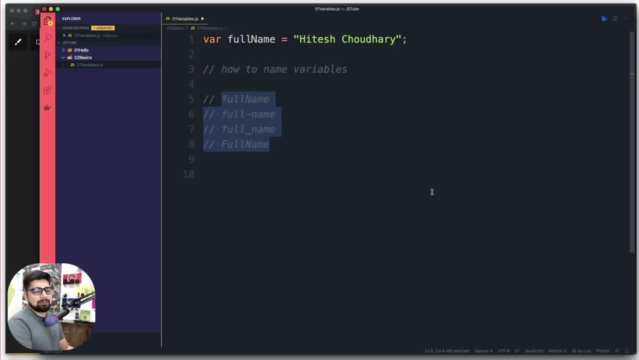 quickly toggles on these comments on and off, so for vs code and most other editors, so fun thing. moving back on to our talk that this is a variable, so i have. moving back on to our talk that this is a variable, so i have revealed that this is a variable. so i have revealed. 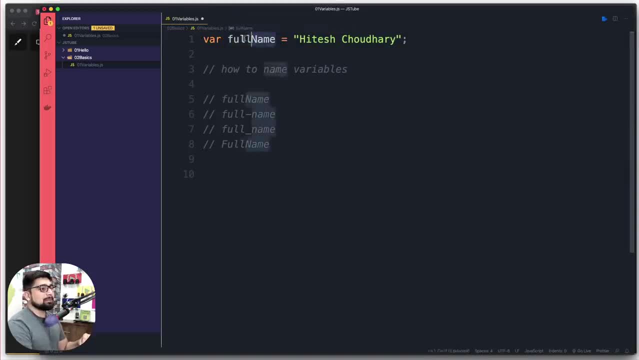 revealed some memory inside. i have reserved some memory and i'm calling that memory as full name, and that full name actually points to this data that i have stored in the memory. now, javascript. we got a whole lot of things that we can do. let's do a couple of more ones so that we can test out. 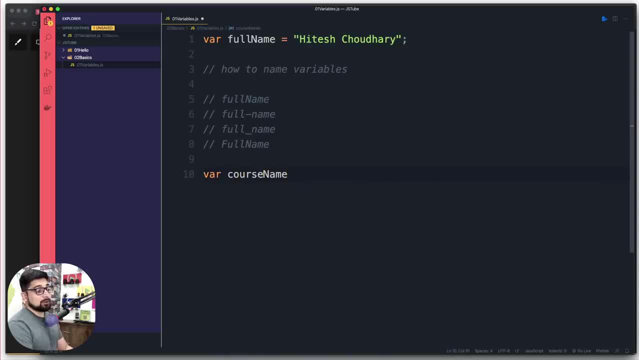 so i'm going to do another one, which is going to be simply course name. of course, at learn code online, we have lots of courses, so we put equal sign and then we define every string or the name that i want to say inside these double codes. for example, i want to say react js boot camp. that's. 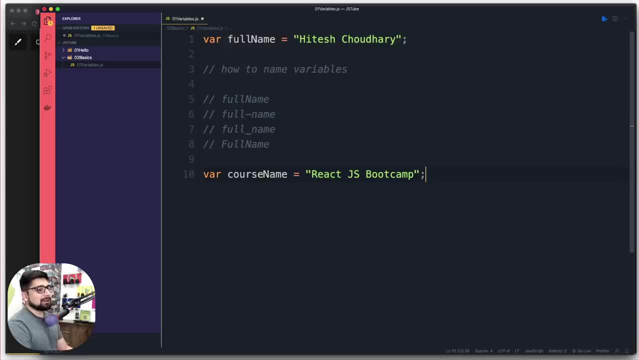 going to go just like that. so now you know how to reserve some strings here. these are strings, of course, but javascript also supports a whole lot of other things. for example, obviously i'm building an application, so there will be people which i would like to check whether they are logged in or not, so 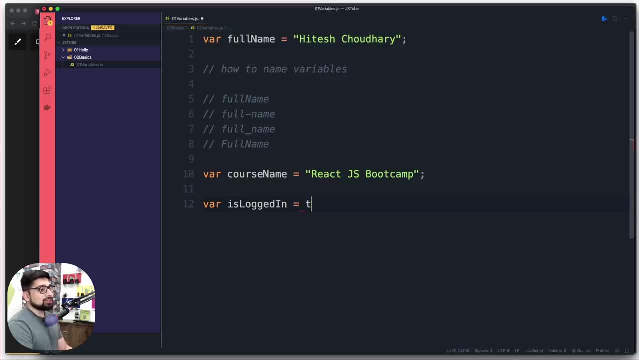 i'm going to say a variable is logged in and i would like to just mark them as true. now. these are known as boolean types of value. there are just two booleans here, true and false. so that's it. that's true and false. so that's it. that's all i've indicated. they're heavily used in the javascript. 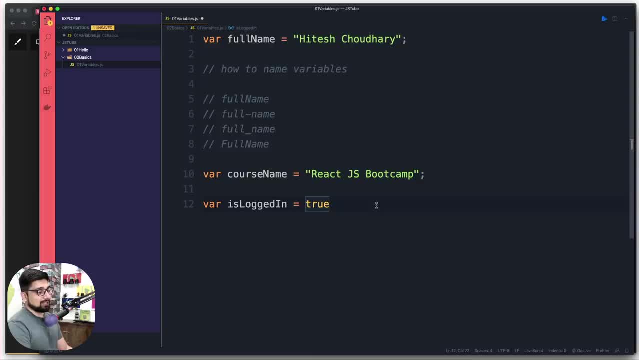 and you're going to see them scattered all around every single place, so you can either mark it as true or you can mark it as false. again, a big thing to remember for beginners. the falls that i've written here and this falls are two different thing in the world of javascript: the smaller. 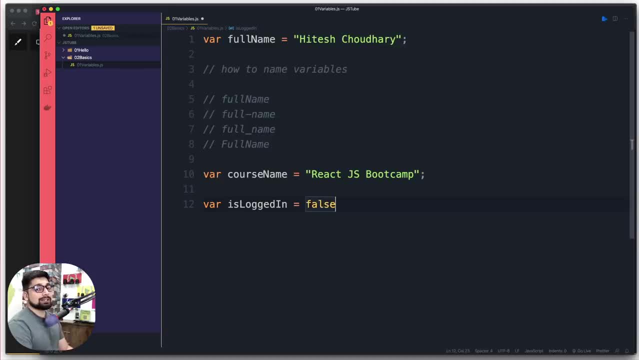 false and smaller. true, that means these are reserved keywords. they have a very specific things to do, basically a switching flip and on. so false simply means it's zero and one means it's true loosely, not one hundred percent, but we just say it like that. okay, put up a semicolon. that's one another thing. and since you're building, 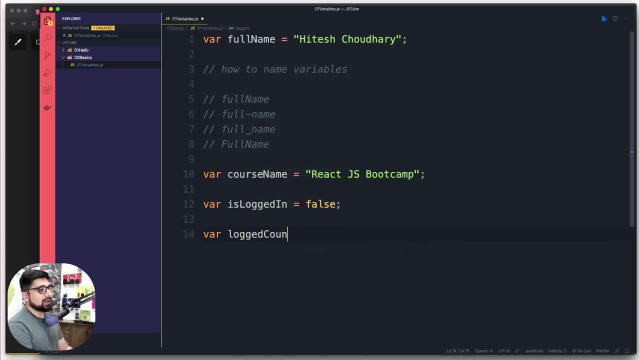 enough application. you also want to check out that how many times users are actually logging in into your application. so let's just say the logged count is 34, some user. there we go, so we can define the numbers here. now. great thing to notice: here only string goes inside. 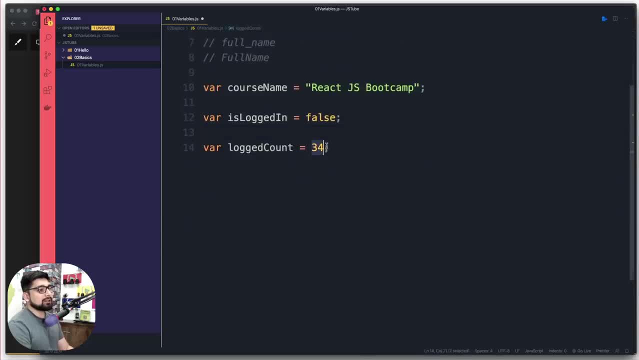 the double codes. so what you are seeing here, the 34 and, if i just wrap it up with the double codes, these are two different things. this is just a string and this is without. the string is actually the number itself. when we do the addition, it becomes a whole lot of mess. so 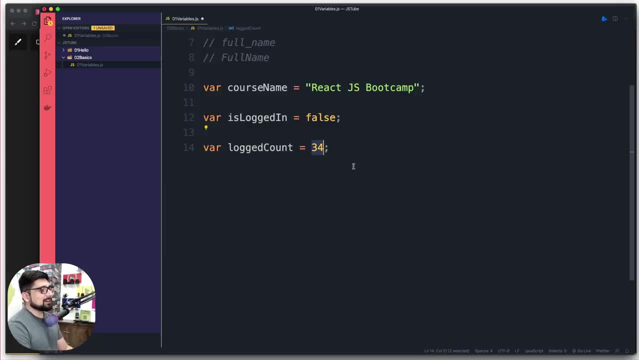 make sure you are aware of it right up here. so these are a couple of things that we are going to have here now. obviously, these are the just the basic ones. what also? you're going to see that sometimes you want to declare a variable. let's just say somebody wants to do some payment. 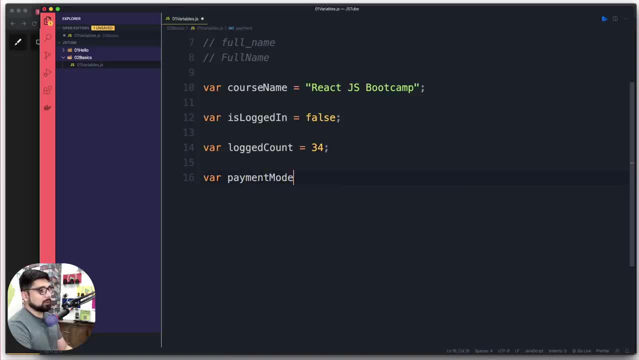 so i'm going to, i'm going to call this one as payment mode and i'm not putting up any value because i don't know what value is going to come inside this one. anybody can pay with credit cards, debit cards, bank directly, so i don't know. later on, when my application runs up, then i would like. 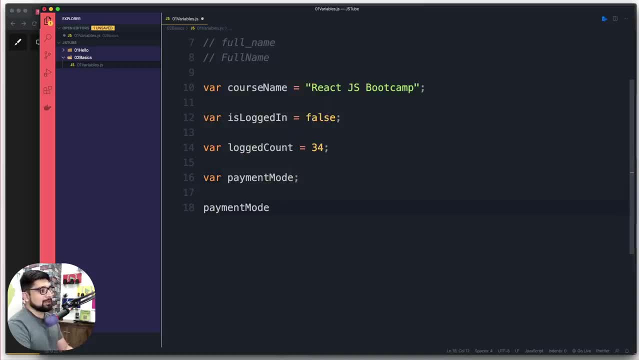 to just add some value on it. so i simply go ahead and say payment mode is going to be simply credit card. so in this time i don't put this war keyword here, because it's already a memory which is reserved, so no need to reserve it again, just use it for the next time. now there is another thing. 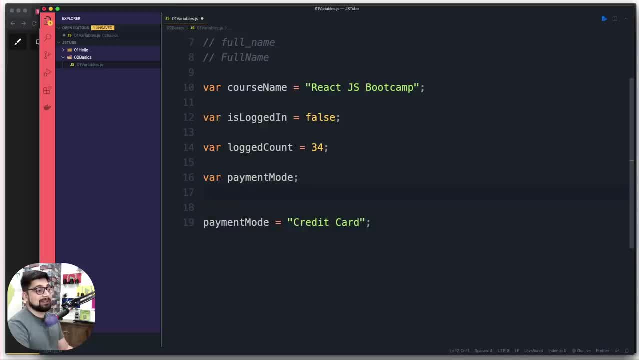 that you are going to see up here. let's do some console log- the very famous thing in javascript- and see some of the things. first and foremost, we're going to do a console log here, so i'm going to simply say a console log of logged this one logged count, so let's go ahead and copy paste this one. 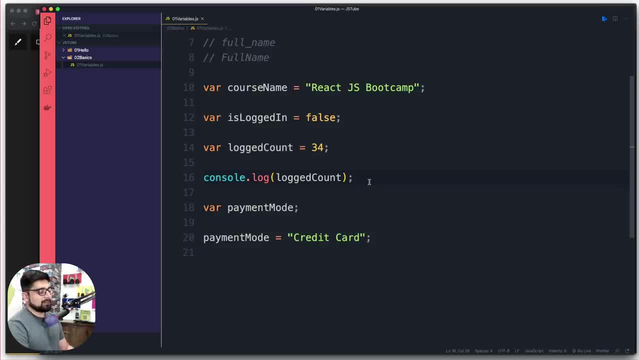 now notice here there is a difference between the two things. first, if i make a duplicate of this and i just wrap this up inside the double codes, this double code simply means i want to display this as it is, without double quote means i'm referring to a variable whose value should be. 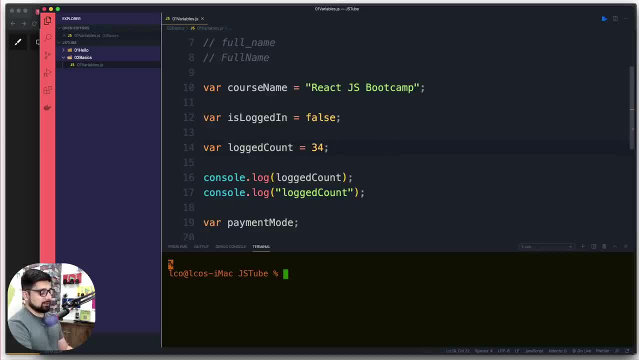 displayed. let's go ahead and save this one and see how this is going to run. so we're going to simply say: node, i'm going to go inside zero, two basics and run this file, which is zero, one variable, dot js. notice here first time it says: 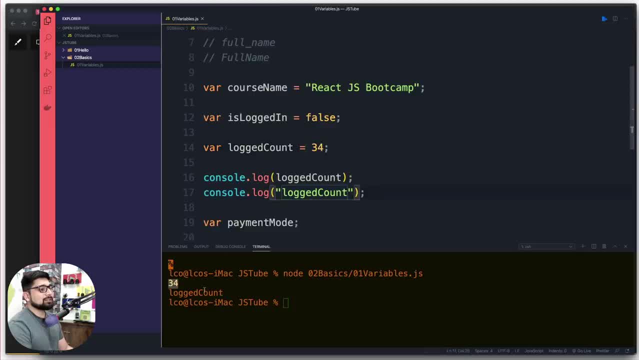 34, because that's actually the value, and the second time it just says logged count. so that's it is okay. so this was all basics. now let's just quickly comment that out. how do we did that? we simply go ahead and say control slash or command slash. that's it pretty easy. 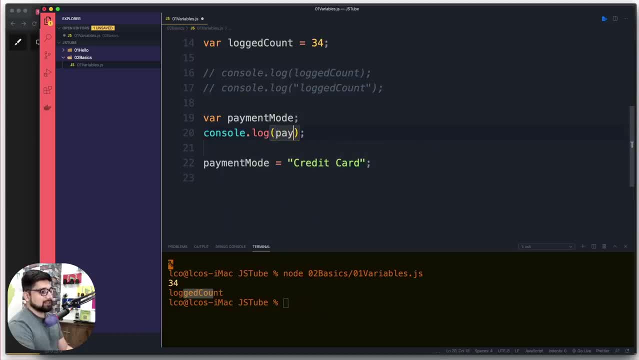 now let's see what happens when i do a simple console log on this payment mode. so i'm going to actually copy this and paste it up here now. you'll be surprised to know that there is another data type that we have to discuss. here. we have discussed how strings are stored, how these boolean values are stored and how 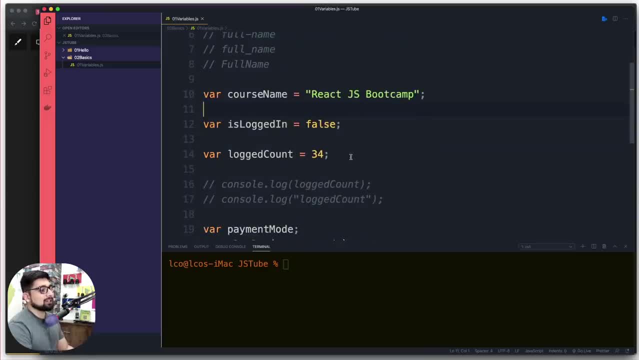 numbers can be stored. there are a bit more. as we are going to get more friendly, we are going to use them. but notice here, something strange is going to come up with the payment mode. there is a memory which is reserved but there is no value inside it. so in such cases, you're going to 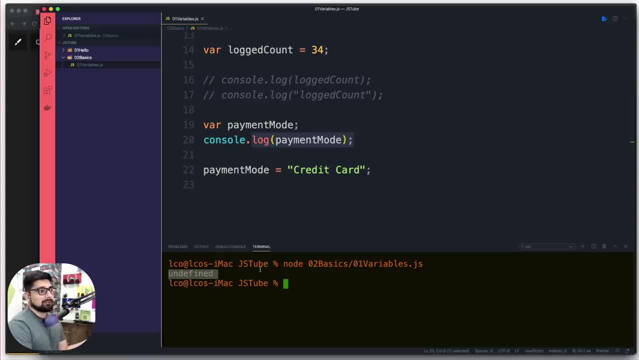 this undefined a lot and in fact we do a lot of case checking with the undefined things as well. so notice here once this is being done, that's how it is. but if i move this one here just below, so notice when i save this and run it this time, this time it's going to give me a value. so yes, 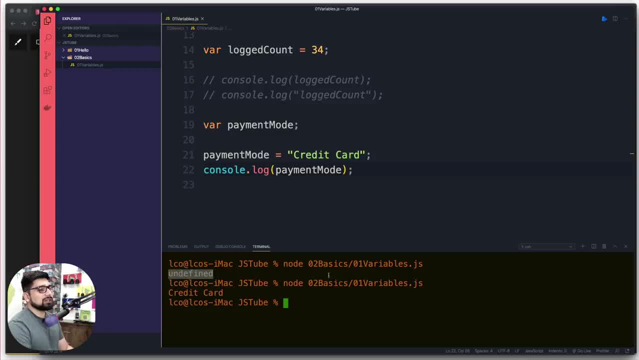 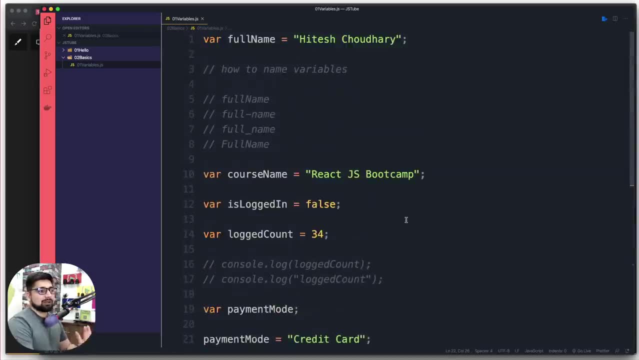 there is another data type here which is undefined. so in total, how many data types are there? in fact many. i don't want to just get you a bother too much right now. just assume there are only these ones. you can store strings, you can store numbers, you can store these boolean values and if you, 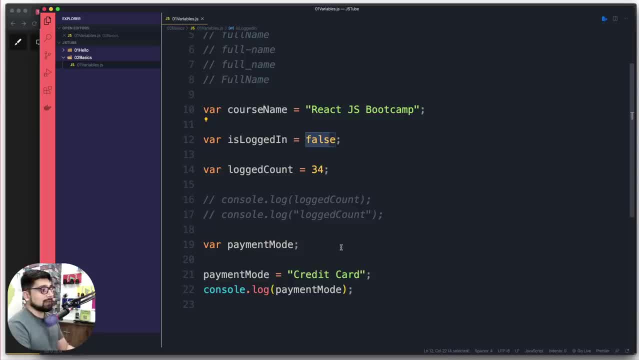 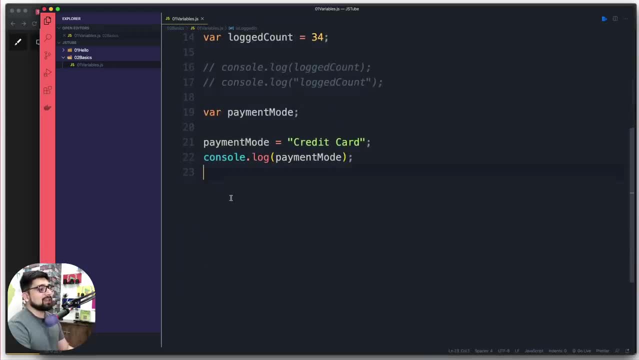 don't store anything that's undefined. eventually, more are going to come and we're going to have a lot of them. now just on to a side one. uh, we have discussed a lot. just one last note. i would like to mention here that there are some reserved keyword as well. no, you don't need to memorize. 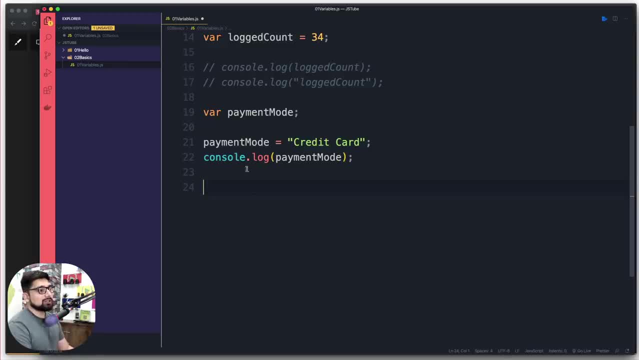 them, but eventually you're going to learn them automatically. so you saw that they. i have this console being appearing in some different colors similar to this. there are some things which are reserved. for example, if is a reserved keyword. so if i just say more, if is equals to 23, i cannot do that. so how do you? 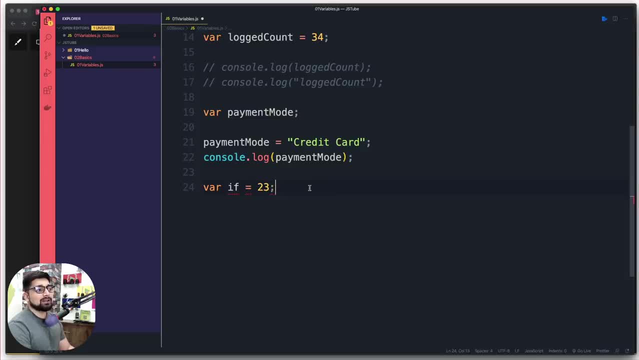 are going to find that if is a reserved keyword. obviously good editors are going to give you some of these hints, just like these errors, quickly bar if you are still writing on the text pad. i don't know why you are just making extra pain for yourself, but let's just say: use good editors. 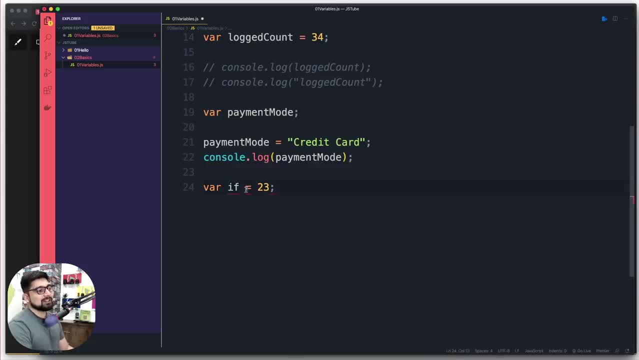 and eventually, by the time you will be finished watching this series, you're going to realize that, yes, there are some reserved keywords which i cannot use. so, quite a lot of discussion, which is why i am here today and i'm going to show you some of the things that you can do to make your 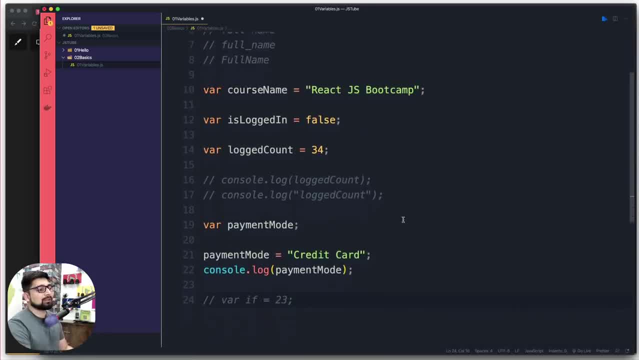 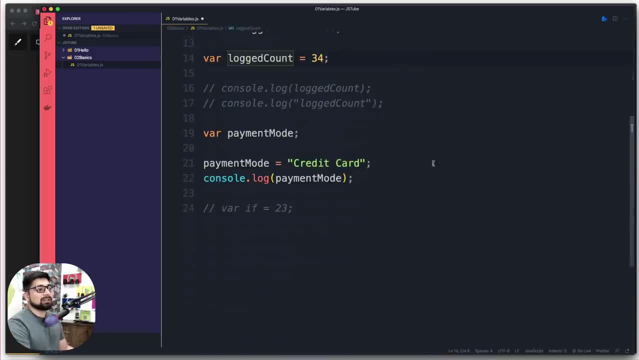 code easier. so if you are a user, of course, name, login count, login count, which was fun, and we were able to at least somehow declare our learn code online application. now we can take user's name course name, login count, logged count as well, as we can define the payment method as well. so i think